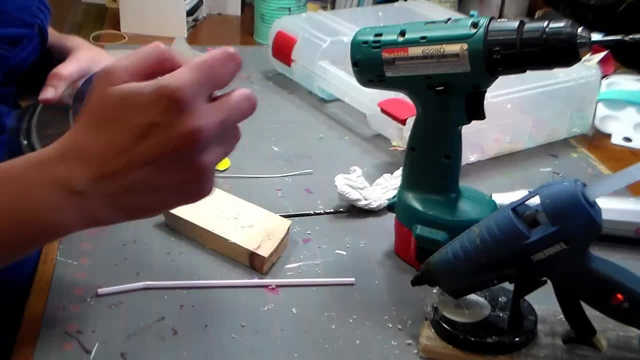 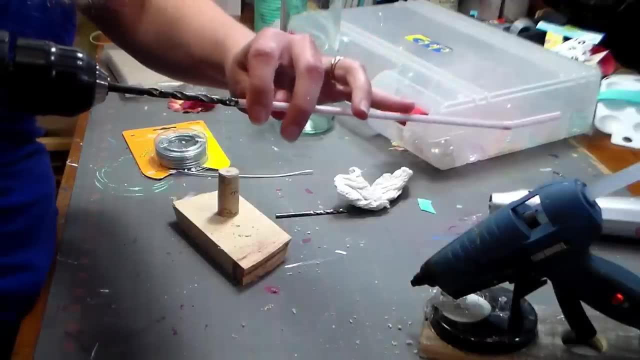 wine bottle and make sure you've washed the cork in the wine bottle well with hot soapy water and rinsed it out really good. Drill a hole in the cork and I'm using a bit that's like the exact same size as the straw. it's like I can't put. 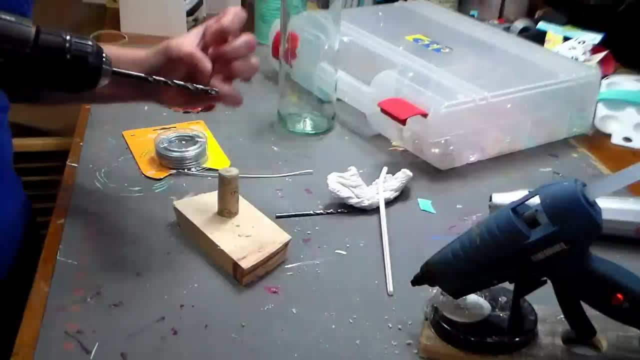 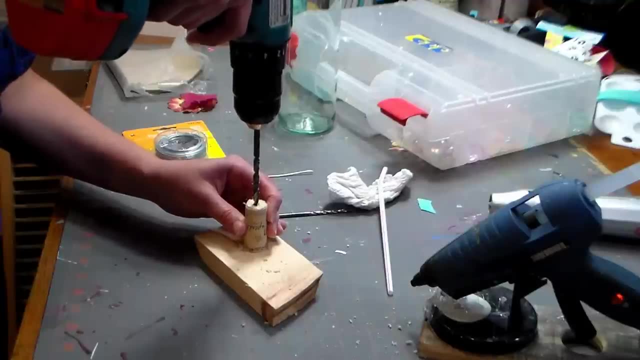 that straw over it. it's gonna the the rubber will kind of contract back in. This is a rubber cork, not a cork cork, and it will kind of contract back in, so you want to make sure that it, the straw, will be able to fit through, and then 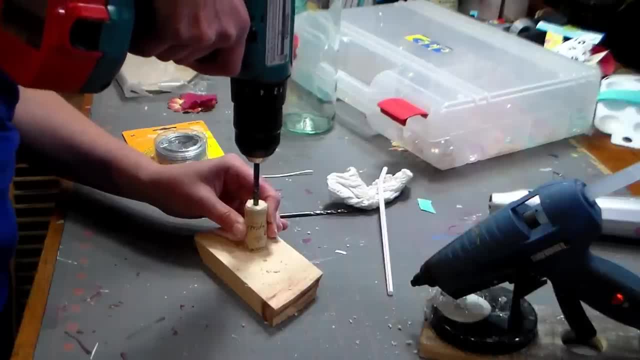 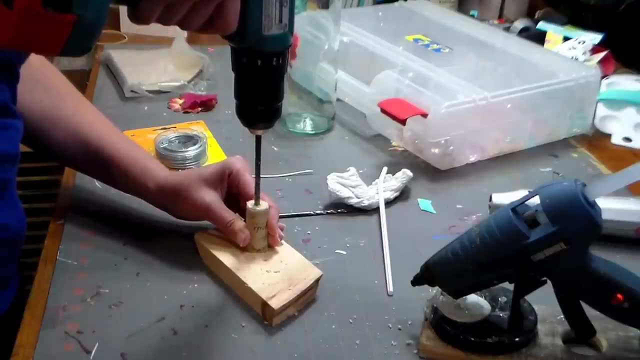 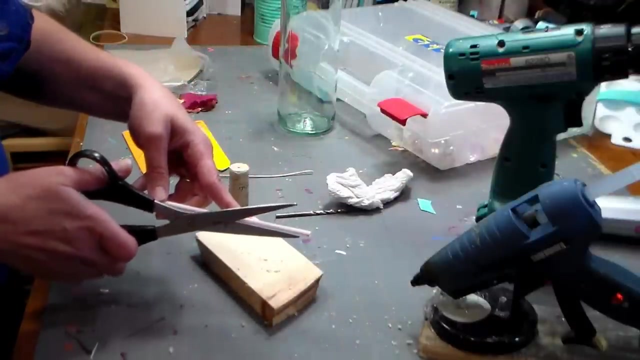 just drill through with your drill. I've done a pilot hole already, so it's going really easily for me. There we go, and then to make the straw fit, you want to cut kind of a long tapered. you want to cut it, cut the straw, so you've. 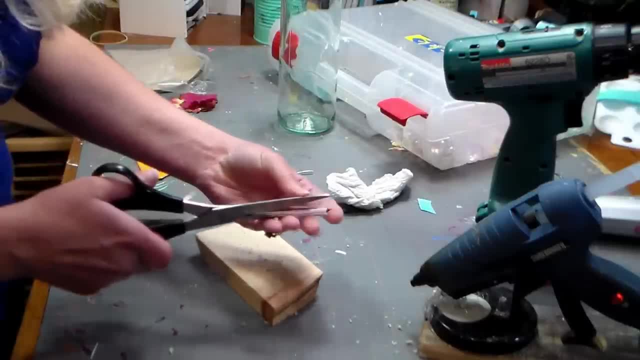 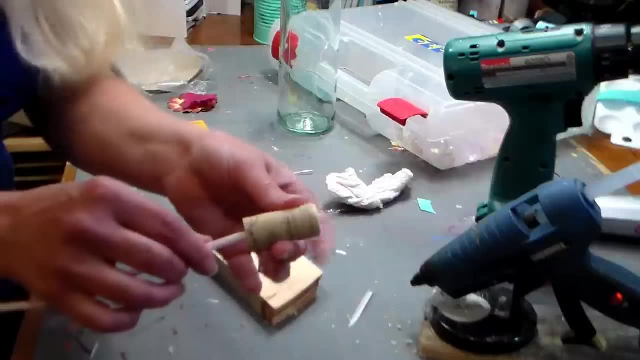 got kind of a long tapered area so it'll be a lot easier to push through, and so I'm gonna go in with my tapered end of my straw. so you want to make sure you cut that taper long enough so it can poke out the end, and then you're gonna 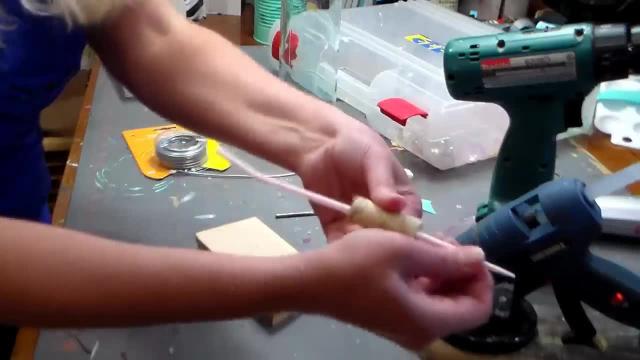 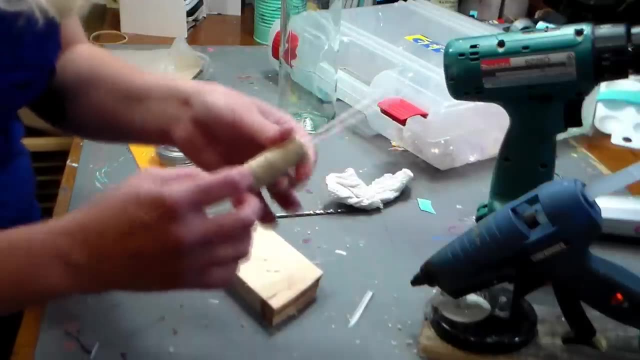 pull it through, okay, and it's really tight in there, okay, so I know it's not gonna leak. so then I've got about a quarter of an inch above the bend in the straw right there showing through. To seal this up, I'm going to use hot glue. 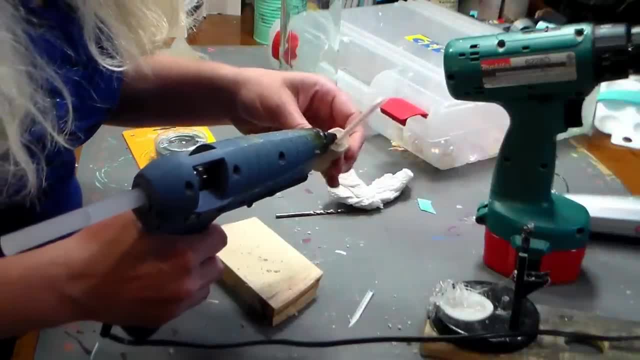 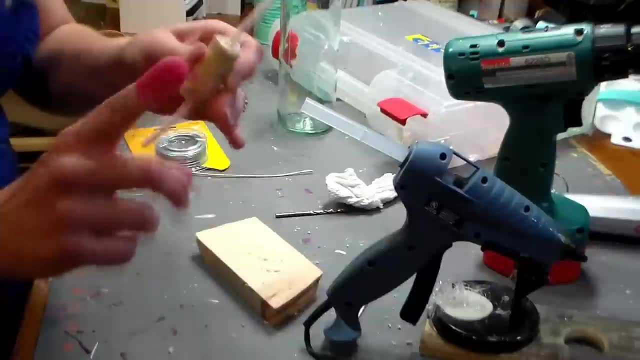 alright. so I'm just gonna do like a bead of hot glue. I'm kind of trying to put it on the rubber right next to the straw so it doesn't burn or melt my straw. I'm going to use this little finger cot. actually I could do it up here. I'm going. 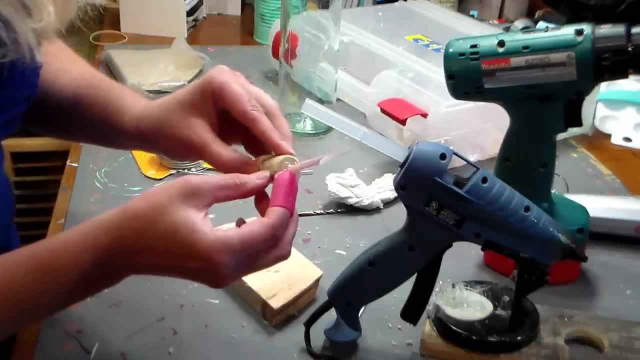 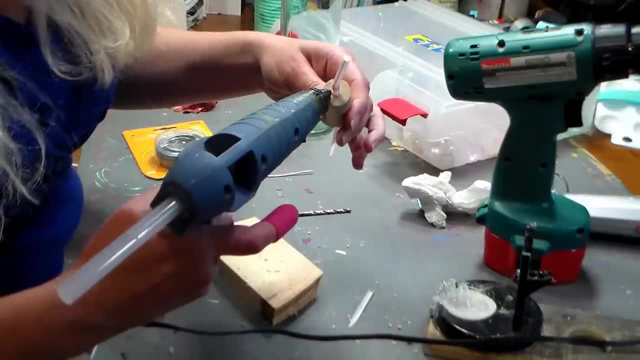 to just press it in there and then I'm going to pull it through and then I'm going to do the same thing here on the part that's going to be seen. so you want to be kind of careful to have it neat and I'm just gonna smooth my finger. 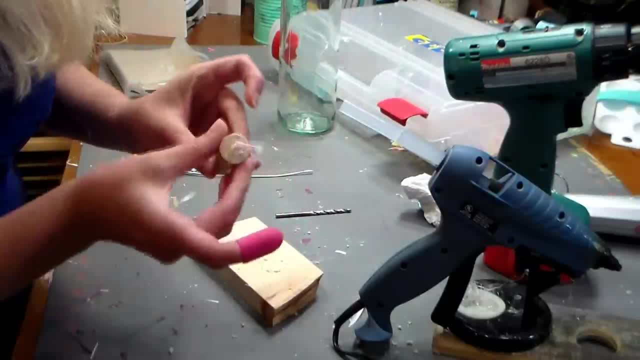 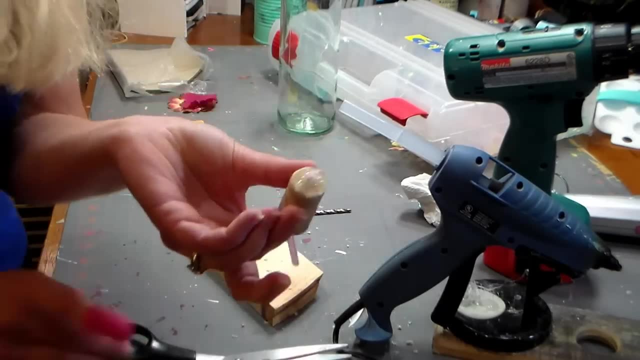 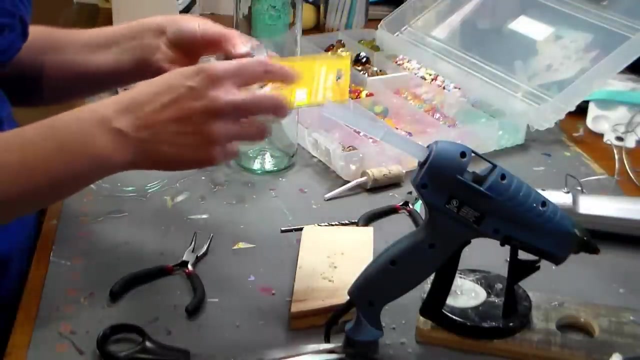 around there just to seal it in so there's no bubbles or gaps. Oh, we will trim this. I'd go about a quarter of an inch there To make the hanger. you're going to want some wire and I'm using 16 gauge steel galvanized wire so it won't. 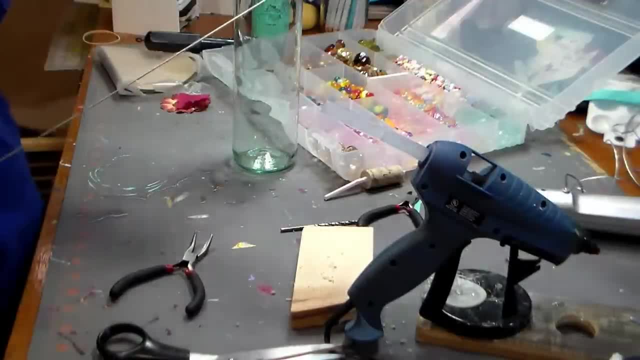 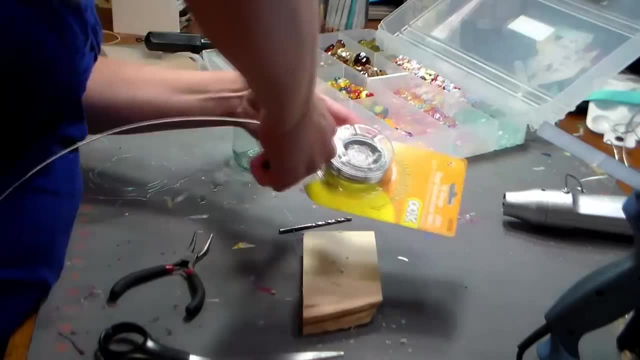 rust and I'm going to use a 16 gauge steel galvanized wire so it won't rust and I'm going to pull off about 4 feet. I learned it's better to have a little extra than not enough. I can cut these with my just standard diagonal pliers here. it takes a. 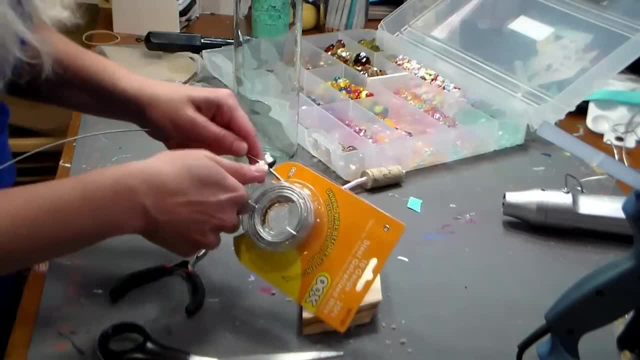 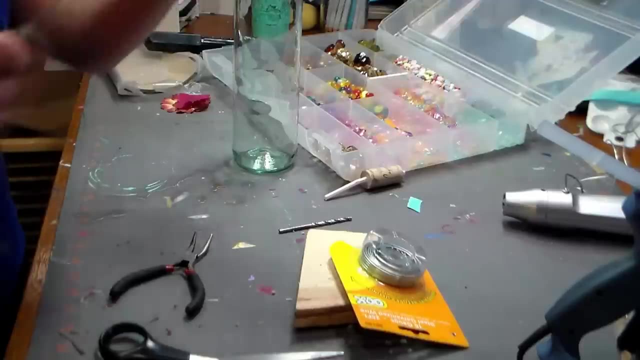 little elbow grease- but I can do it- and some of these actually have little cutters on them. paint those chintzy little cutters. Now, what I'm gonna do actually is find the midpoint of my wire, which is about 4 feet long, and I am just going to make my hanger here. so I've got the end. 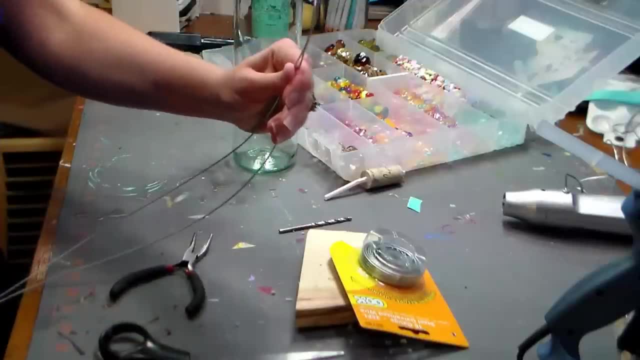 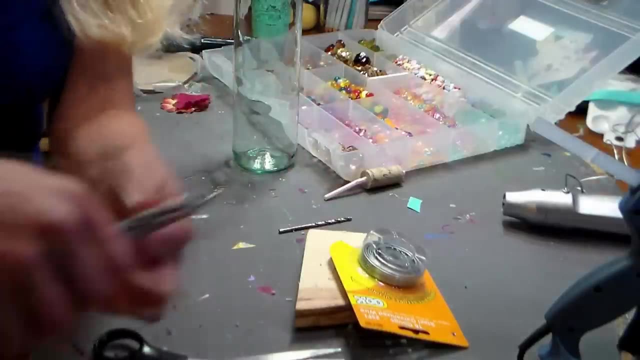 and I'm just gonna twist it and actually I'm gonna grab that with my pliers. anyoure that you like to use are fine. I got my dinky little jewelry ones. probably your manly man pliers will be better for this, but this is gonna be just fine for. 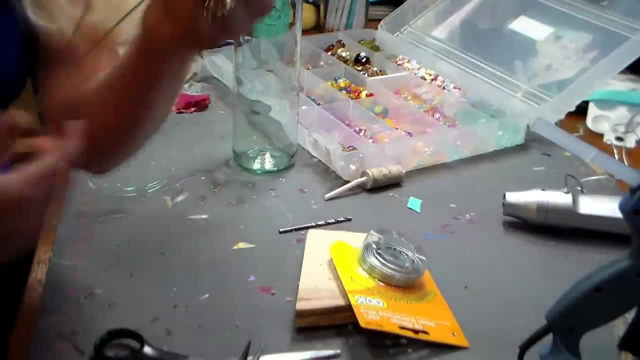 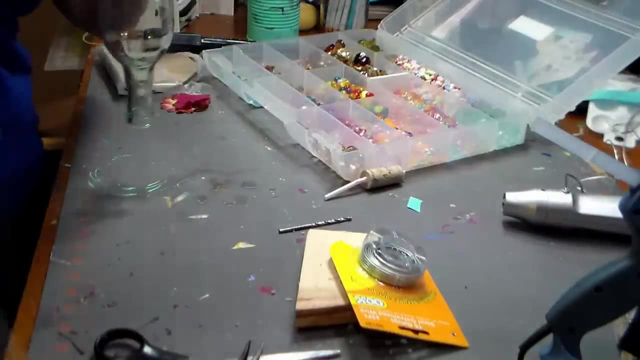 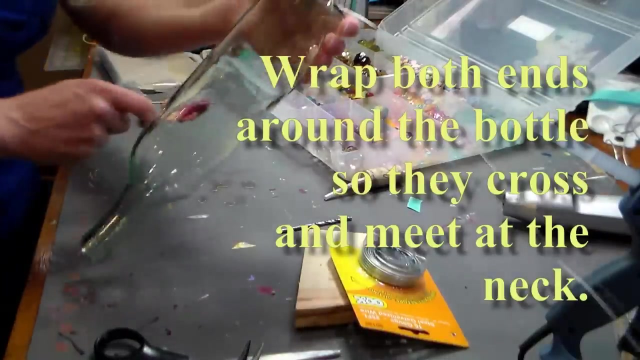 me and I'm gonna give it a couple twists, okay, and that's what you'll hang that with. I'm gonna bend it so that's gonna be kind of right at the end, right in the middle, and then I'm just gonna start wrapping the wires around my bottle. 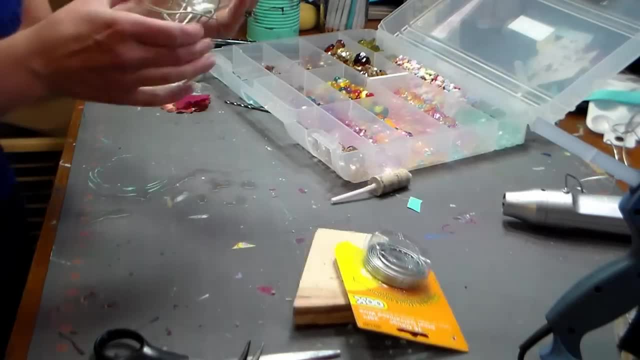 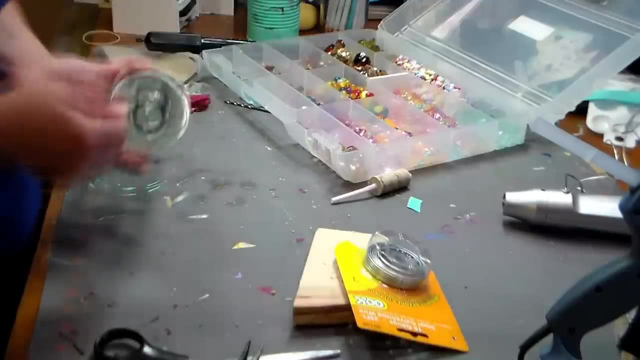 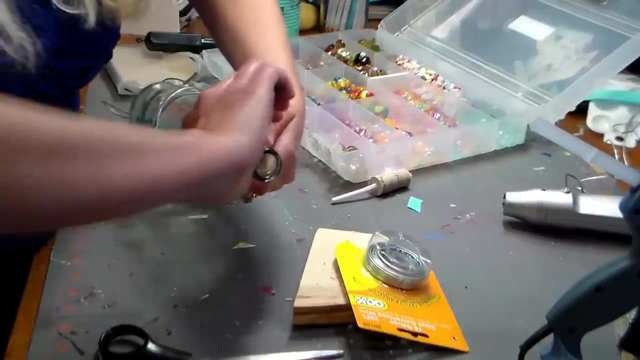 Okay, I'm gonna leave that tail right there, okay, so at the bottom where they meet, I'm gonna grab them, together with pliers and twist, and this is incredibly awkward. so if it doesn't feel natural, then you're probably doing it right, Okay? 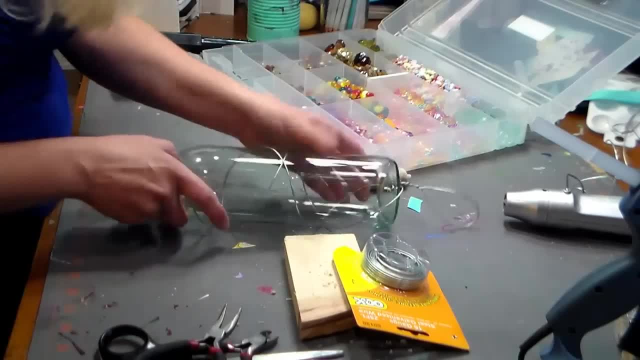 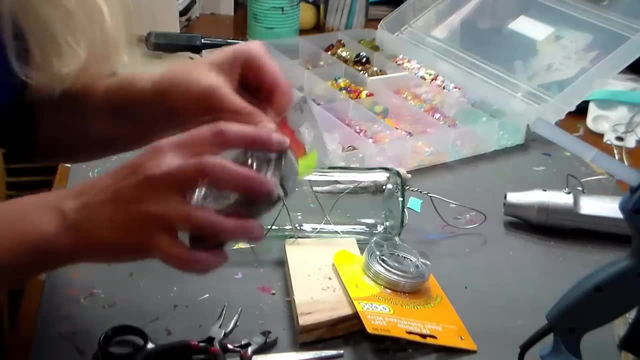 so what I'm gonna do now is get some thinner wire that I can add some decorations with, and I'm gonna use 18 gauge aluminum wire and the same wire I used to make the dinky man pliers. higher the number, the skinnier the wire. So now I want to use an assortment of 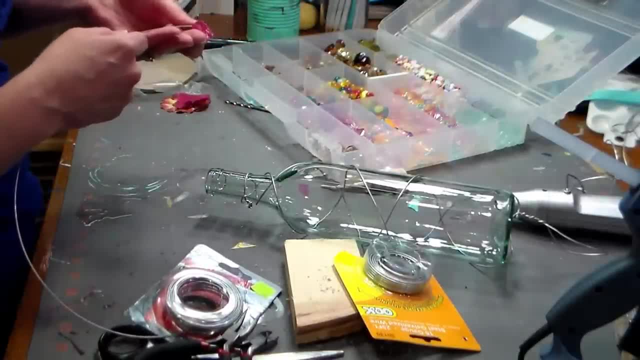 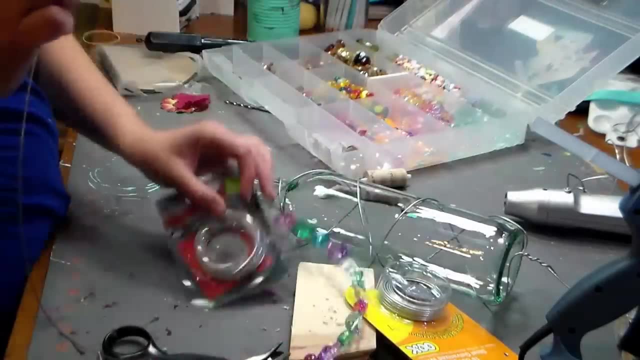 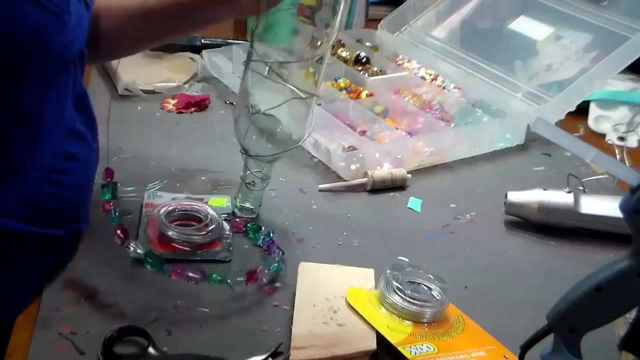 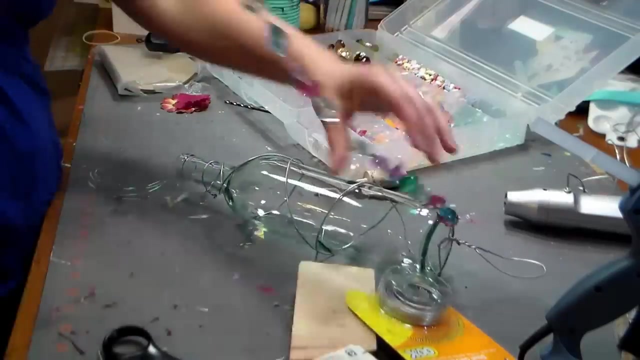 lovely beads that are very sparkly. Okay, we have a strand of lovelies on there, so what I'm going to do now is kind of wrap it up here, wrap it over the center a few times, and I'm gonna wrap and just make sure that as I go I am kind of 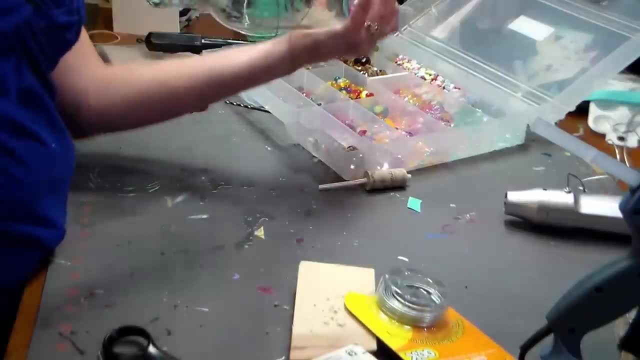 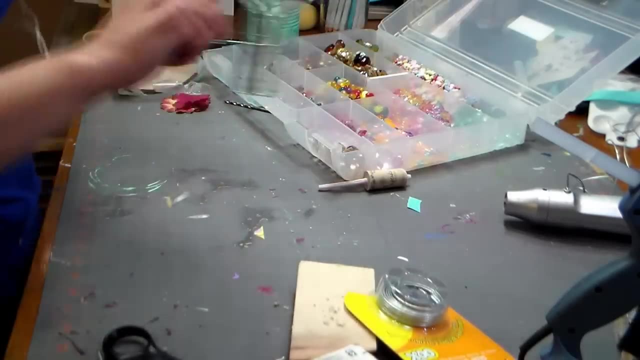 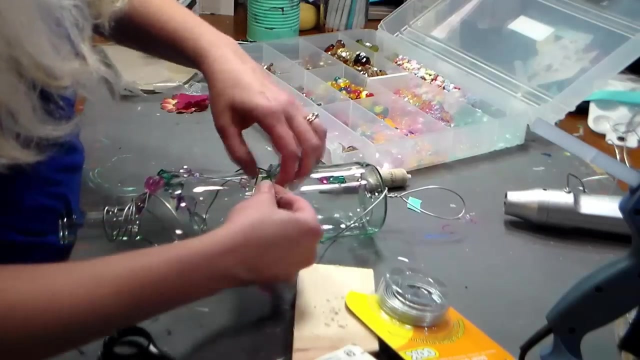 distributing my charms, my beads. Oh, that's so pretty. it's sparkly. I love it. Oh, I've got some little butterflies I could put on there too. It's a light and it will attract the birds, because I read actually that you. 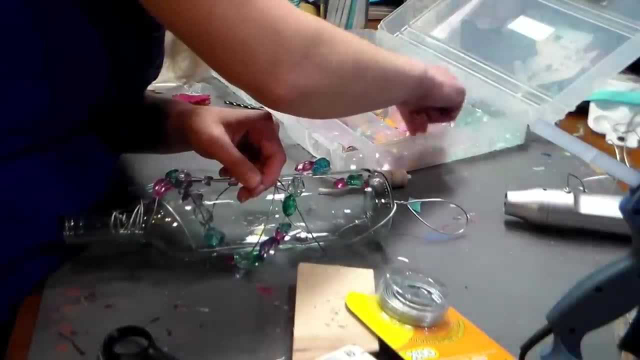 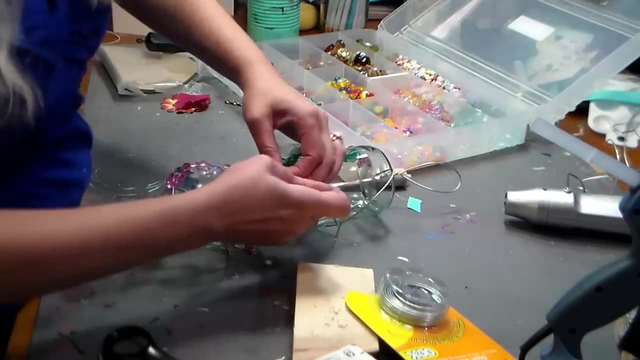 shouldn't put the die in the feeder. that it's not good for the birds. Alright, so I'm just going to go up and wrap right around this one. I should have left even a little bit more, or maybe not wrap it around so much here. 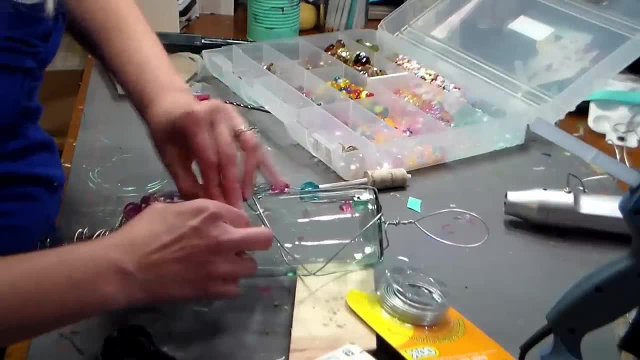 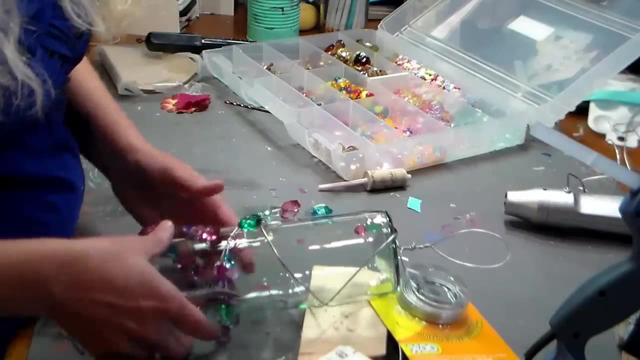 on the bottom. I'm just gonna wrap this little tail around a couple times, Trying to get it under both wires for a little extra stability. There's are forgetful hummingbird feeder Forgot. I want to add a little little clothing to this and I'll do it now. the first step is to do that and again pick up enough lace as I can. 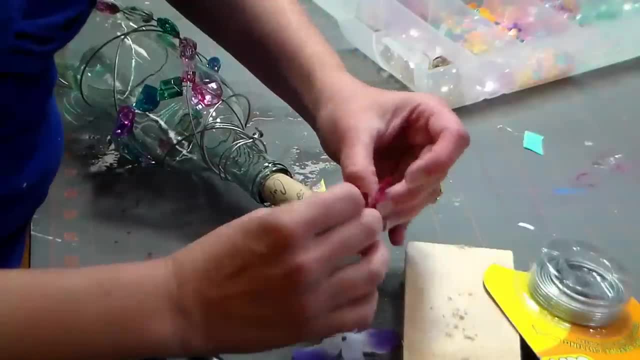 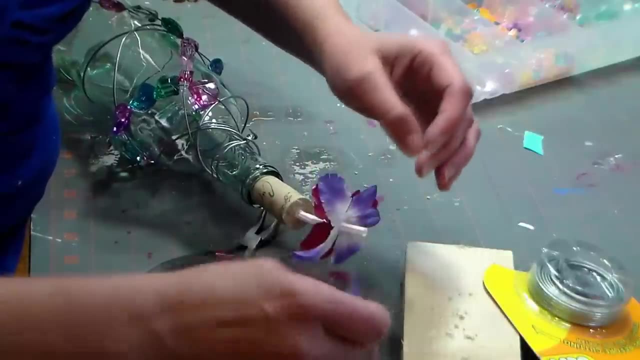 little flower so my hummingbirds know what to shoot for when they're out there looking for food. so I'm gonna take a couple of these silk flowers. I just save silk flowers if, like, we have like Lay's or something like that around, or 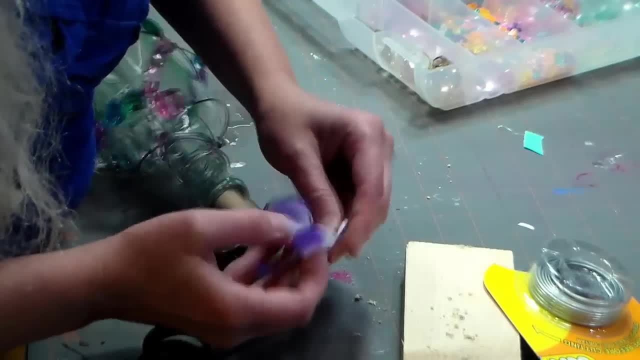 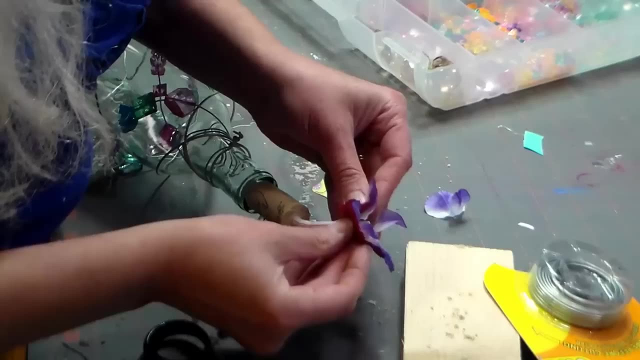 I'll buy them at the craft store or the dollar store and I just cut them apart to use for craft projects. so I'm actually just gonna glue on. I'll just glue on these two silk flowers there. You could have probably also put like a: 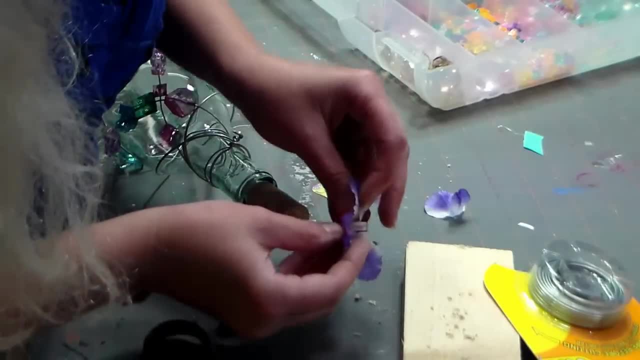 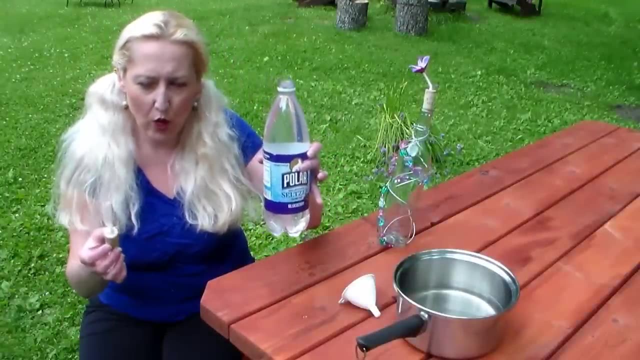 little bit of red wax or something on the end. Okay, I want to share some science with you really quick Now. this is a bottle and it just has water in it. it's a plastic water bottle, My first prototype. my cork was too big to fit my 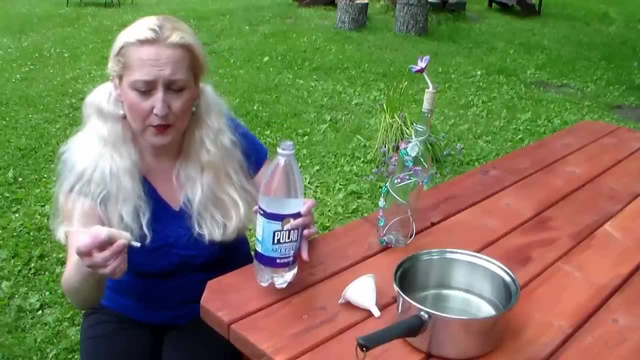 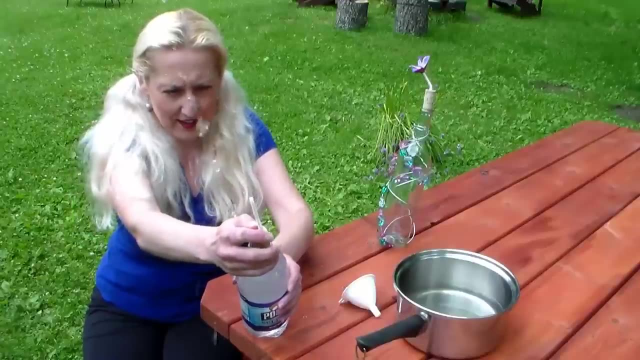 glass bottle, so I thought I would just try it with this plastic one to see. and yes, you can use a plastic bottle. so I filled this right to the top just with plain water, just for the sake of this lesson, and I'm gonna put that in there. 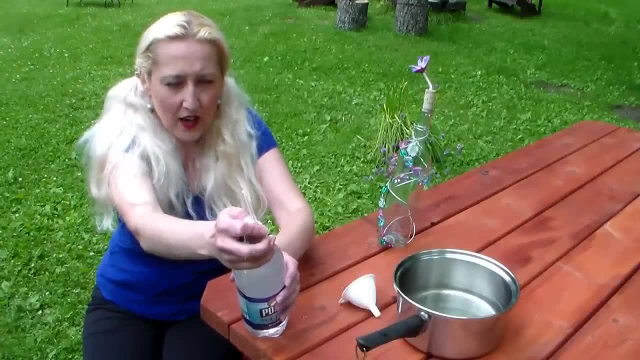 and look, oh, it just kind of spurts out because I have a little too much in there. but I want to talk about why it's so important to have a plastic bottle, and I'm gonna show you why. this just doesn't leak all over the place. A vacuum is formed when we do. 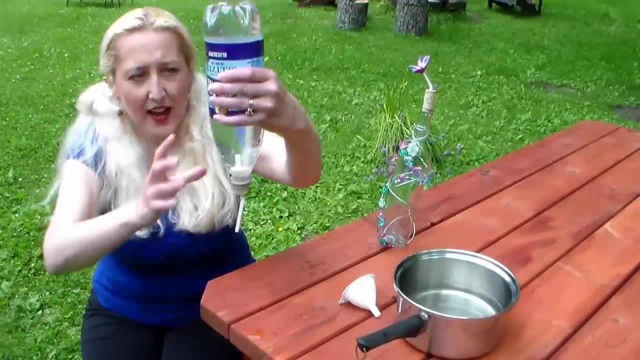 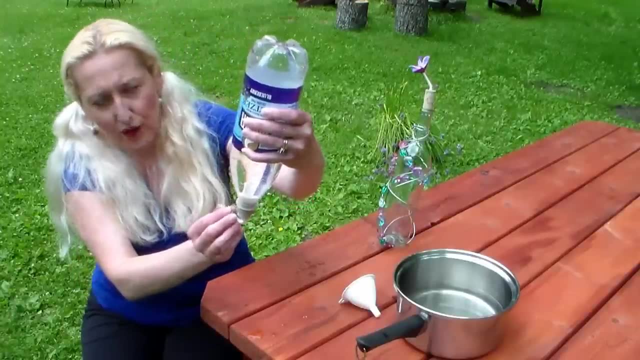 this. so if I have this like this, all the way full, and if this is glass and you can't squeeze it, the hummingbird's not gonna be able to get anything out of this because it's going to be. there's too full and I don't know if you can see. 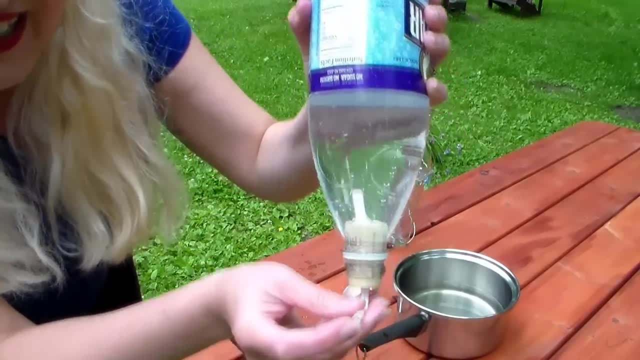 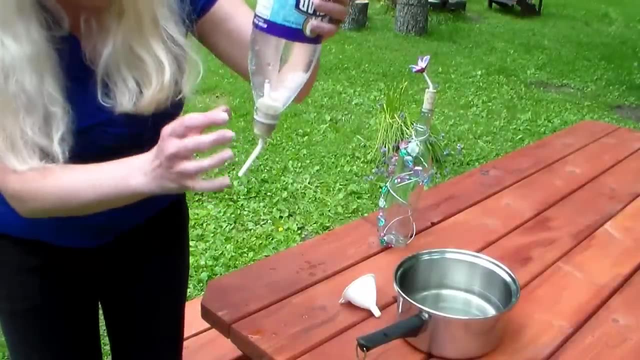 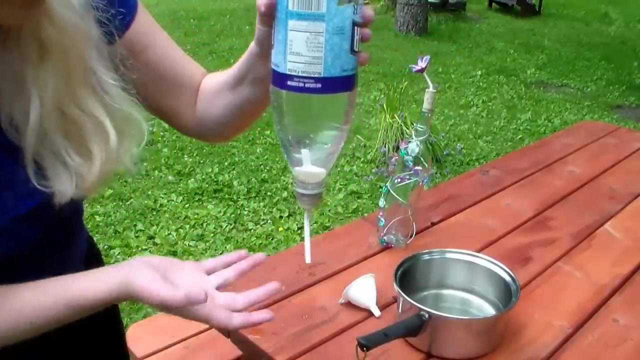 that in the camera, but there's no water in that, in that spout in there. Now I could squeeze it, obviously, and just place the water that way, but even when I let go, you can see the bubbles up there, the water actually the vacuum is up there and there's no water coming through. so you 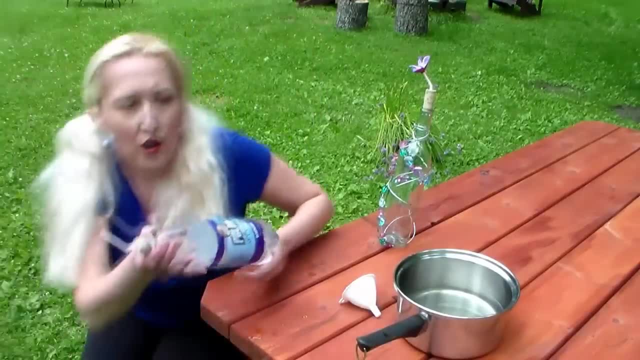 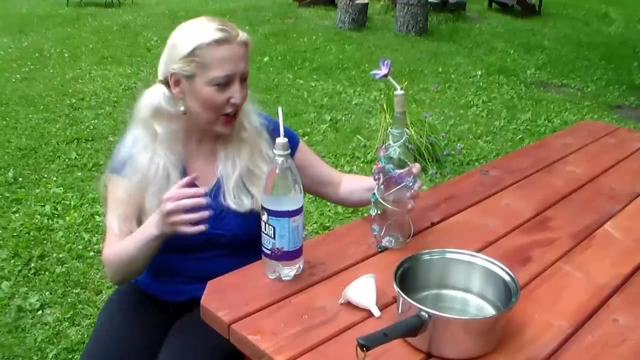 don't want to fill your hummingbird feeder too full. Now if you fill it not quite full enough then it's gonna leak and drip, so you kind of have to get that happy medium. Now I have my feeder here and I have kind of pushed the wire.